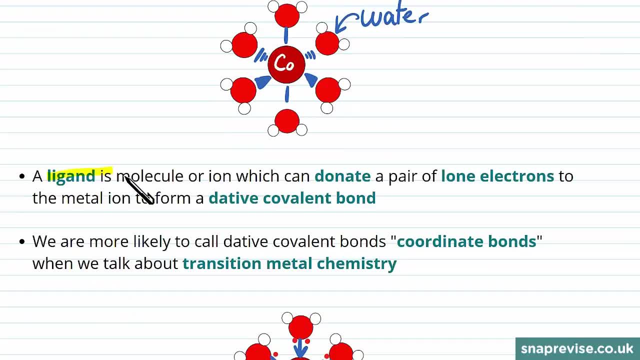 So what is a ligand? Well, a ligand is a molecule which can donate a pair of lone electrons to a metal ion and form a dative covalent bond. Remember, a dative covalent bond is where we have a covalent bond between two atoms, but one of the atoms provides both of the electrons for the 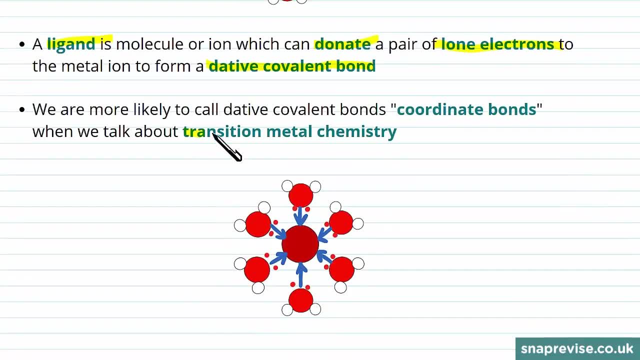 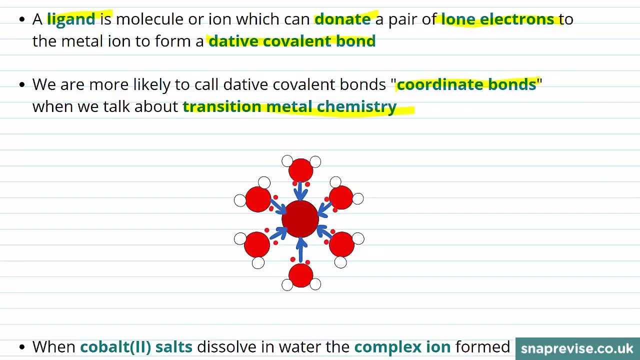 pair. When we're talking about transition metal chemistry, we're more likely to refer to these dative covalent bonds as coordinate bonds. So now we can fully describe a complex ion. It's a central transition metal ion surrounded by these ligands, which in this case are water, and they donate these. 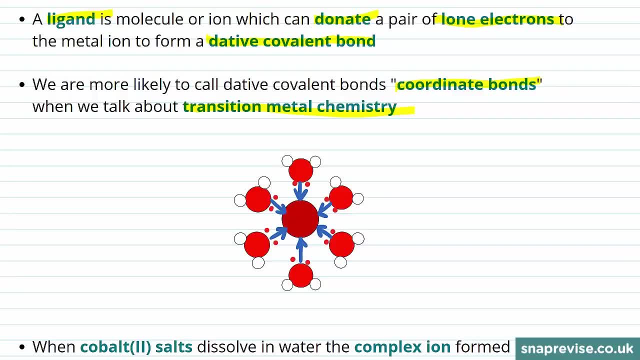 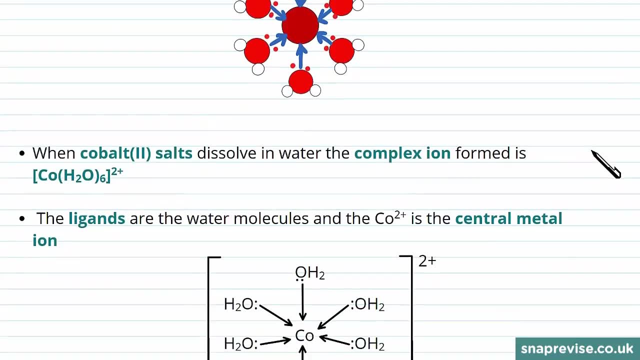 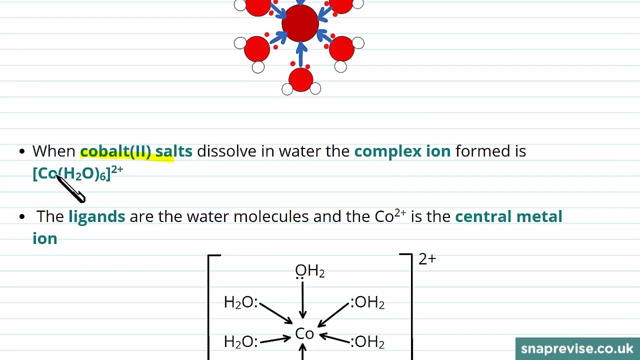 lone electrons to the metal ion to form covalent bonds, which we call coordinate bonds, because the ligand provides both electrons. Subtitles by the Amaraorg community. cobalt salts dissolve in water. the complex ion formed is cobalt CO, and then 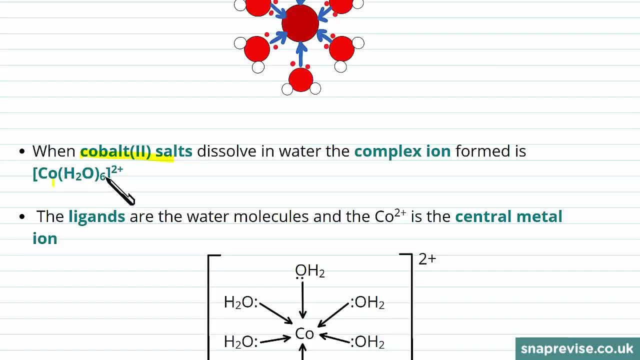 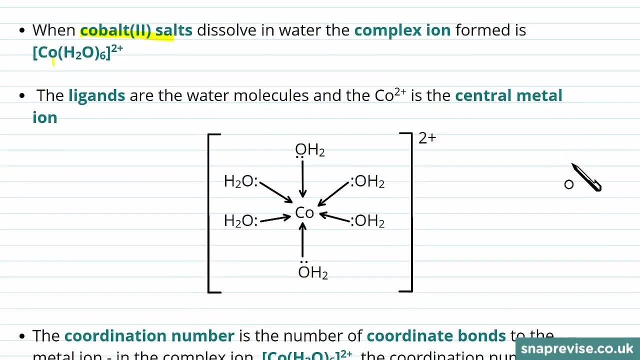 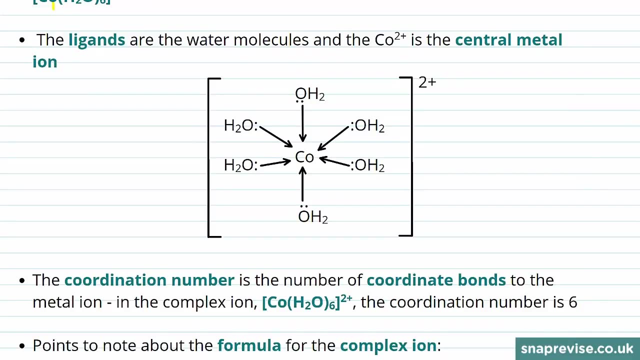 in brackets. we show the ligand and how many of them- there are six- and then the square brackets here indicate that it's a complex ion and we show the charge outside the brackets. so just to break that down again, we often show complex ions in notation like this: we have the central metal ion, which is cobalt. we 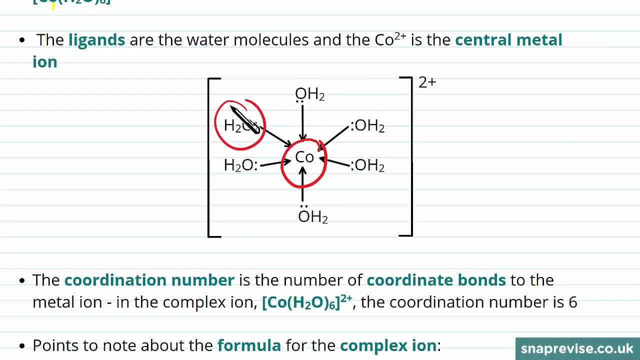 have the ligands showing their lone pairs, which in this case are the H2O molecules, and the arrows pointing inwards show that it is a dative covalent bond or a coordinate bond. we have these square brackets to show that it is a complex ion and the charge is shown outside the brackets in the top. 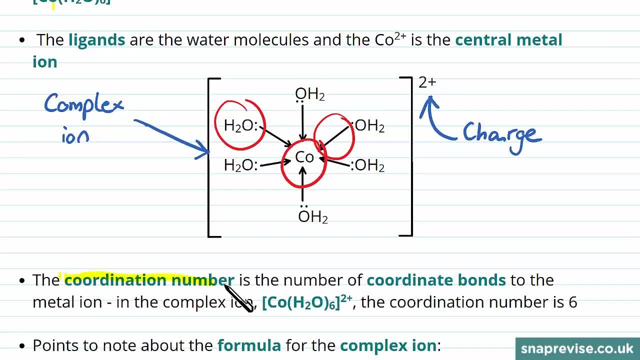 right hand corner. another term we must understand is coordination number. this is the number of coordinate or dative covalent and the charge is shown outside the brackets in the top right hand corner. bonds to the metal ion. so in this example above we have one, two, three, four. 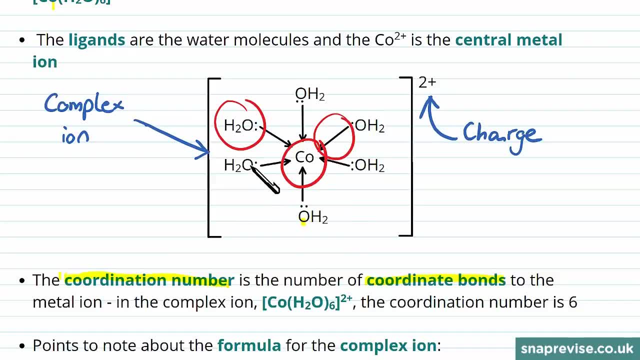 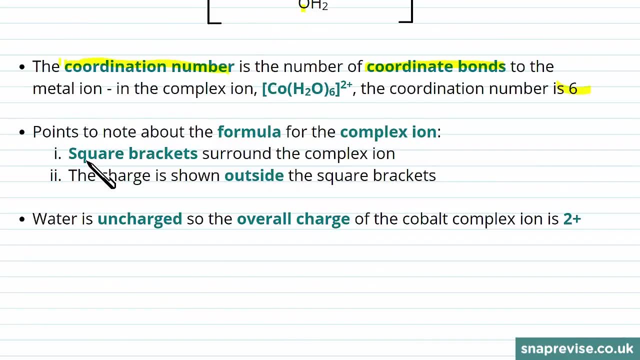 five, six dative covalent bonds, so this complex has a coordination number of six points. to note about the iron that we've already talked about, the square brackets which mark it out as a complex ion and the charge shown outside of these square brackets, water is uncharged and so in the example of cobalt above, 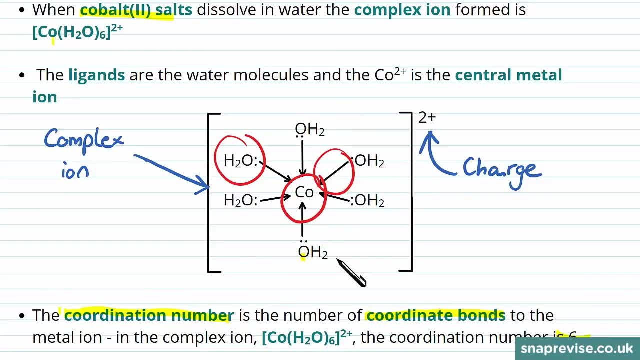 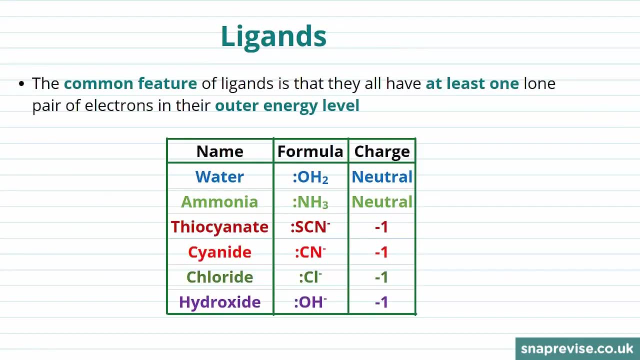 the cobalt has a two plus charge and this gives the overall charge to the complex ion, because there's no contribution from the water. when we look at some other things that can form ligands, the common feature that makes all of them ligands is that they have at least one lone pair of electrons per 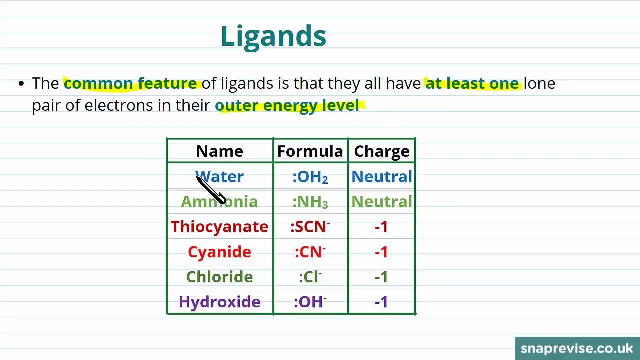 molecule in the outer energy level. so we've already seen water in the previous examples acting as a ligand. but ammonia also has a lone pair. these two, water and ammonia, a similar sizes and they're both neutral. some other common ligands are thiocyanate, SCN minus. 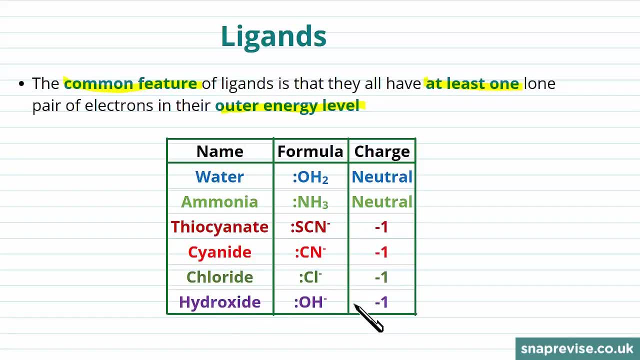 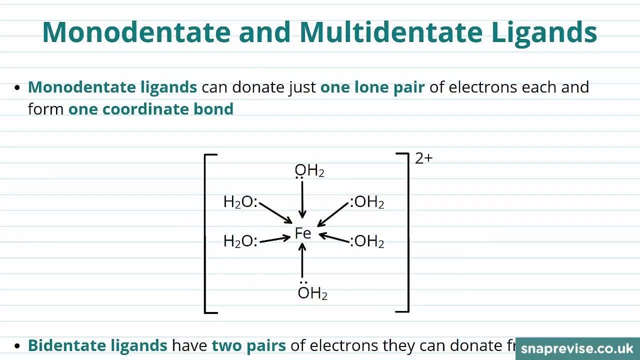 cyanide, chloride and hydroxide, all of which have a negative charge and, as we'll look at more in the future, chloride is bigger than water or ammonia. we can divide ligands into different categories. monodentate ligands can donate just one lone pair of electrons and form one coordinate bond, in fact. 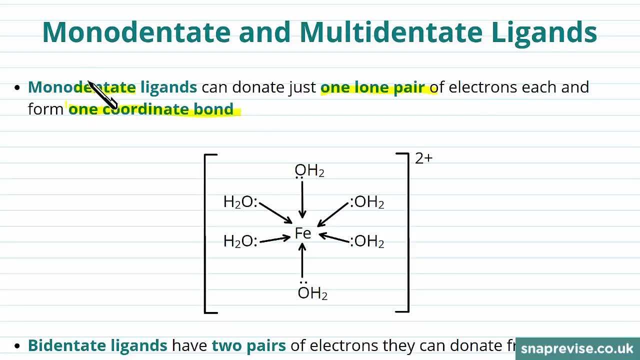 the dentate part of monodentate comes from the Latin of tooth or to bite, and mono means one, so monodentate would have originally meant one bite, which is showing that they only attach in one place. H2O is a good example of a monodentate ligand and you can see here. 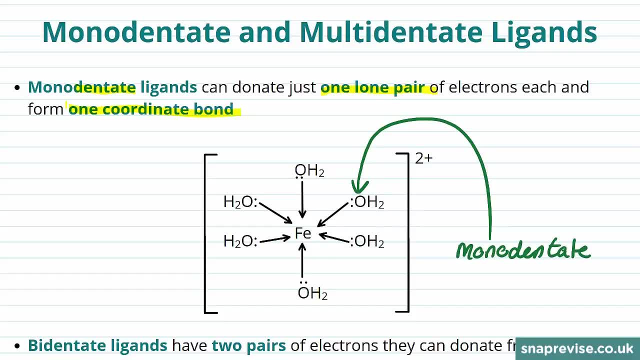 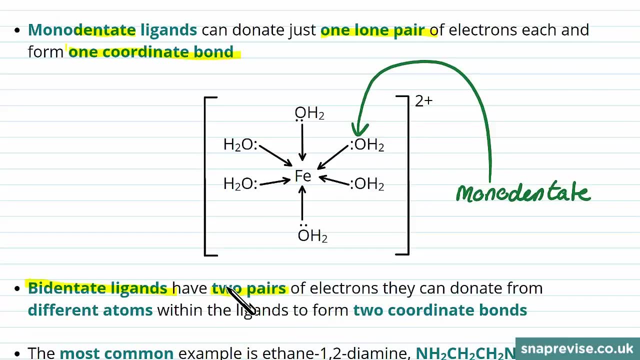 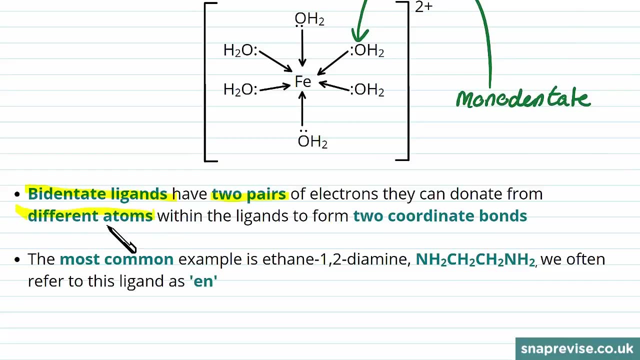 that the oxygen only donates one lone pair per molecule of water that bonds by dentate ligands have two pairs of electrons. they can donate to form coordinate bonds with the central metal ion. these electrons come from different atoms within the ligands, the types of molecules that 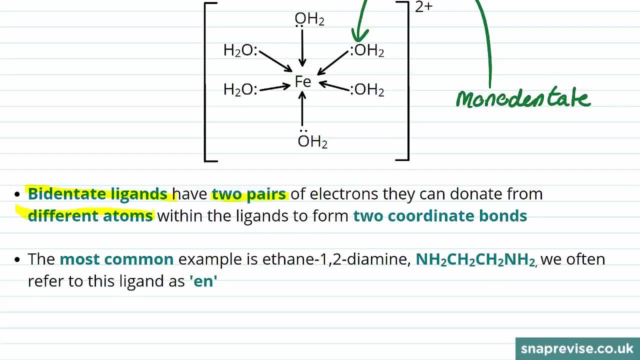 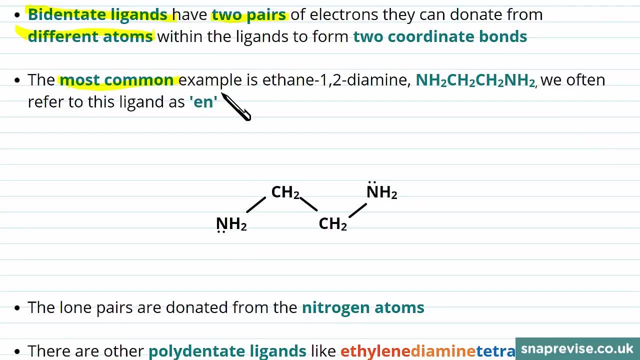 form monodentate ligands, so more than one covalent dative covalent bond you won't have come across so commonly in chemistry. the most common example of a by dentate ligand is ethane one two diamine, which we often refer to for ease as just em when we're drawing out complexes.